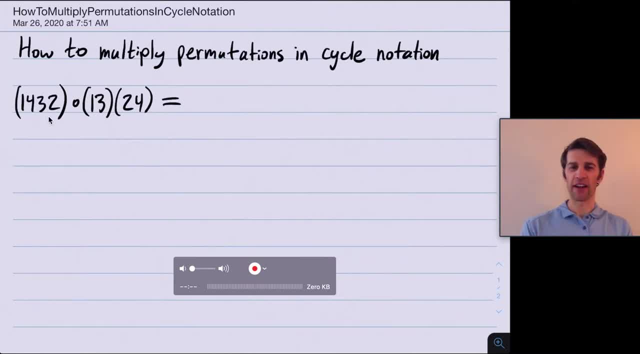 is that we have one function and then following by another function. So let's draw out what each of those functions do. So this first function- 1,, 3,, 2, 4- what it does is it's going to act on the elements 1,, 2,, 3, and 4.. 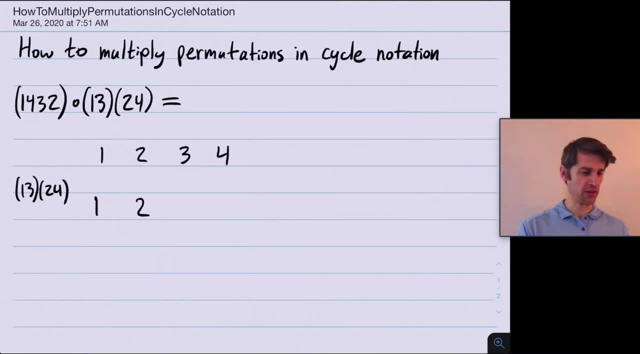 It's a permutation, so it's going to send them to some reordering of themselves and it's sending 1 to 3, 3 back to 1.. It's sending 2 to 4 and 4 back to 2.. Okay, and then. 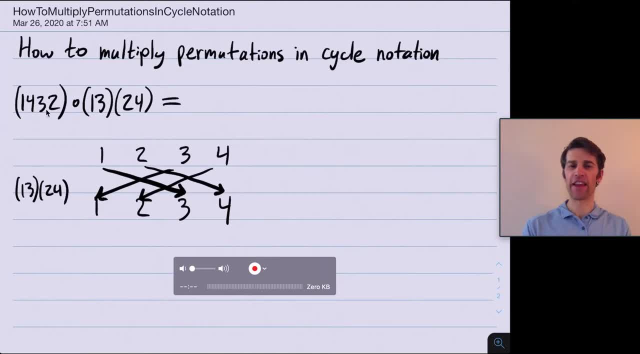 this composition notation means first do this function and then do this function. So what happens next is we're going to do the function 1,, 4,, 3, 2. And it's going to permute these elements 1,, 2,, 3, and 4.. 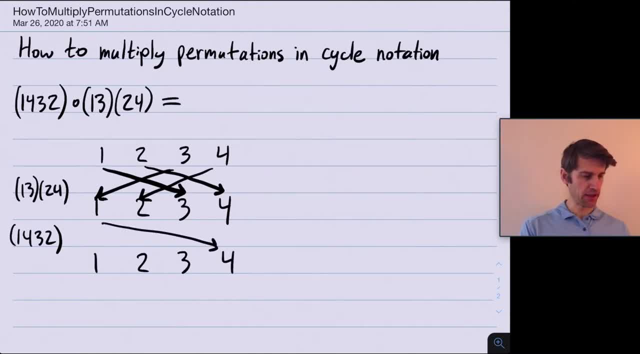 It sends 1 to 4.. It sends 4 to 3.. It sends 3 to 2. And then it sends 2 back to 1.. So the answer on the right hand side. we can already figure out what it should be. 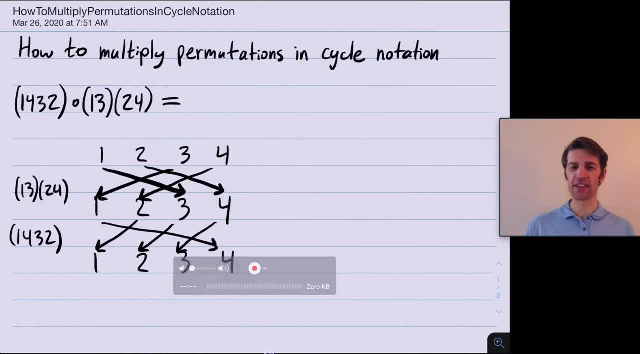 The way we do this is we're going to sort of compose these braids together. We're going to follow 1 all the way down, Follow 2 all the way down, Follow 3 all the way down And then follow 4 all the way down. So what should we get on the right hand side? 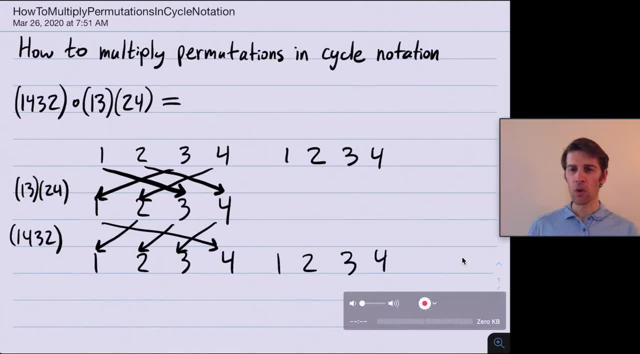 Okay, what is this sort of equal to? Well, 1 is being mapped to 3, which then mapped to 2.. So, overall, 1 is mapping to 2.. 2 is mapping to 4, which is then going to 3.. So, overall, 2 is going to 3.. 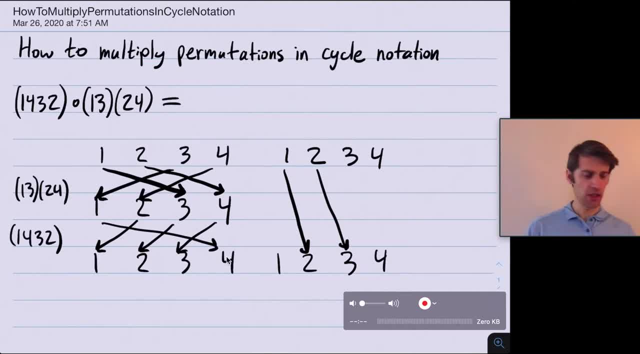 3 is mapping to 1, which is then going to 4.. So overall 3 is going to 4.. And we already know 4 should be going back to 1.. But let's check: 4 is going to 2 and then to 1.. 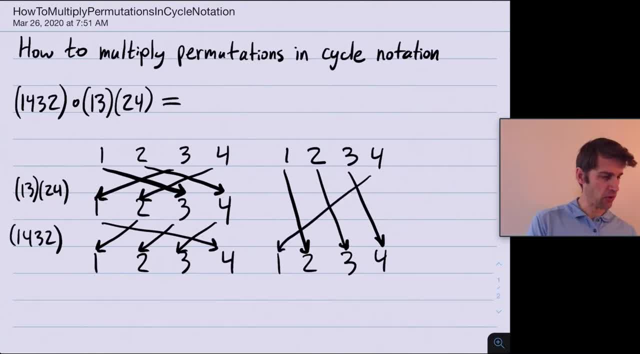 So yes, overall 4 is going to 1.. Okay, so from this picture on the right hand side, we should already be able to guess what the answer is going to be in cycle notation. But let me teach you how to do this Even without drawing the pictures. 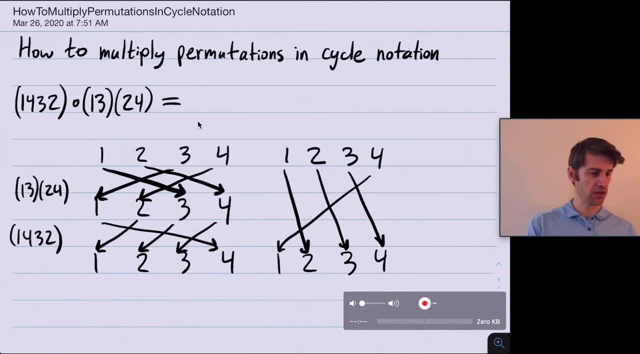 Okay, so we want to see where 1 goes, So let's start off by seeing where 1 goes. Well, this permutation 2,4 doesn't move 1.. This permutation maps 1 to 3. So currently 1 is being 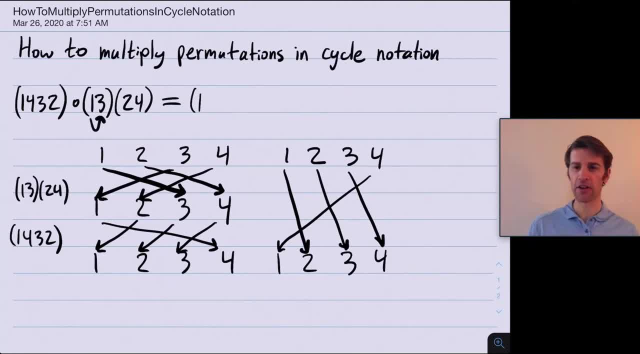 mapped to 3.. I like to draw this with an arrow underneath. And then this permutation takes 3 to 2.. So next, 3 is going to 2.. So where has 1 gone? 1 has gone to 3, which then goes to 2.. So overall, 1 is going to 2.. 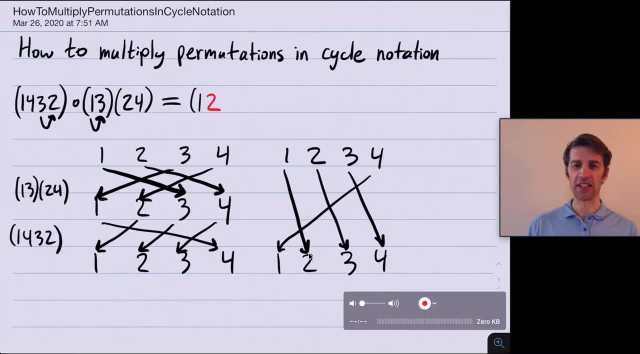 You with me. so far, That agrees with this picture down here. Now let's try to figure out where 2 goes. Well, so first we apply this function and 2 is going to 4.. And then this doesn't move 4 anywhere, And this moves 4 to 1.. 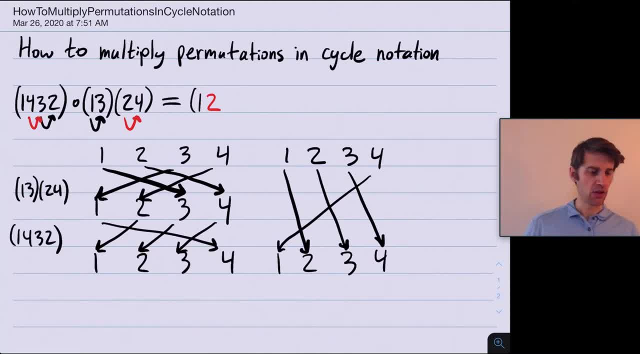 So overall, 2 is going to 4, which is then going to 3.. So 2 goes to 3.. And now let's see where 3 goes. Okay, 2,4 doesn't send 3 anywhere. 3,1 sends 3 to 1.. 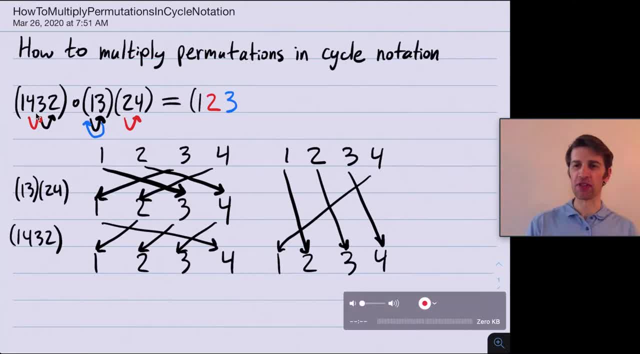 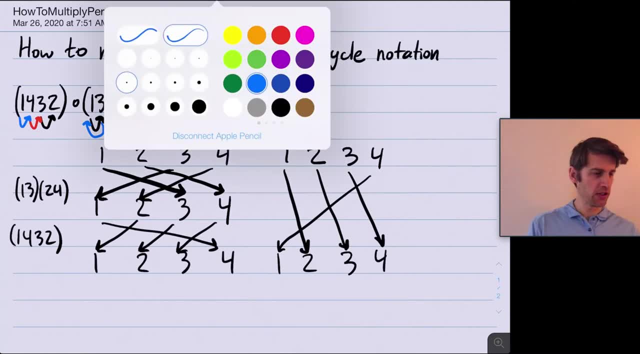 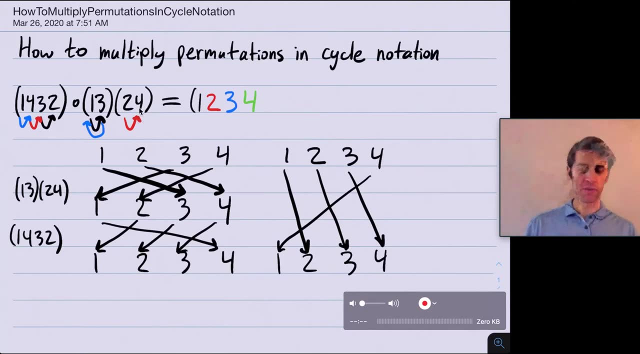 And then this permutation 1,4,3,2 sends 1 to 4.. Okay, so 3 is going to 4.. And finally, let's see where 4 goes. Well, this permutation 4,2 sends 4 to 2.. 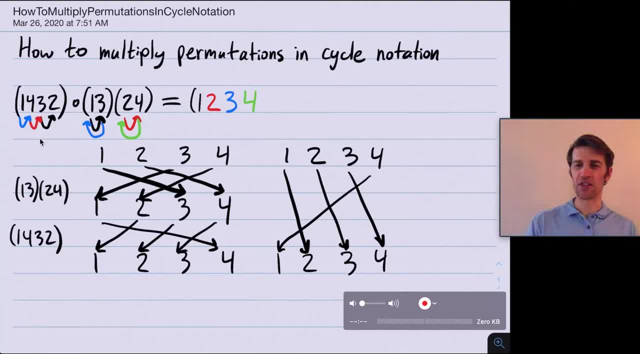 And then 1,3 doesn't move 2 anywhere, And then this cycle 1,4,3,2 sends 2 back to 1.. Okay, four in total is getting sent to two and then to one, since four is getting sent. 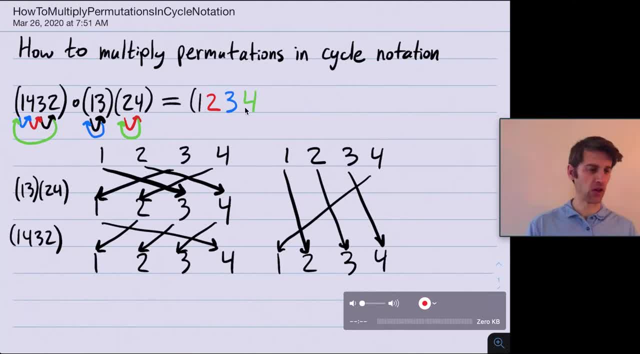 to one to denote this in cycle notation. I just want to close off. the cycle. four is getting sent back to one. okay, so our answer agrees with what we drew out down below. this is indeed the permutation one, two, three, four, four going back to one. but the advantage of doing things as I've done up above is that I don't need 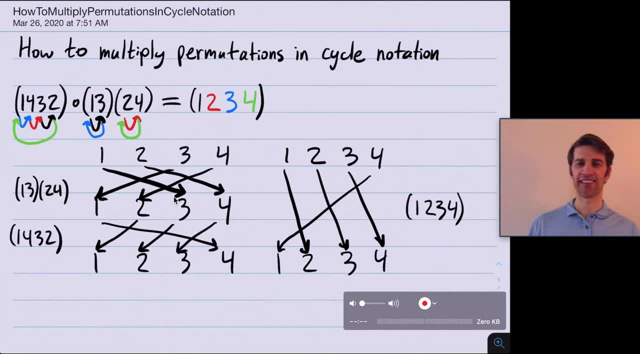 to draw the pictures to get the right answer, okay. one other comment is that you'll note that drawing these colored arrows can help you do this at first. eventually, you'll get to a stage where you don't need to draw those colored arrows, but it's a good practice tool at the 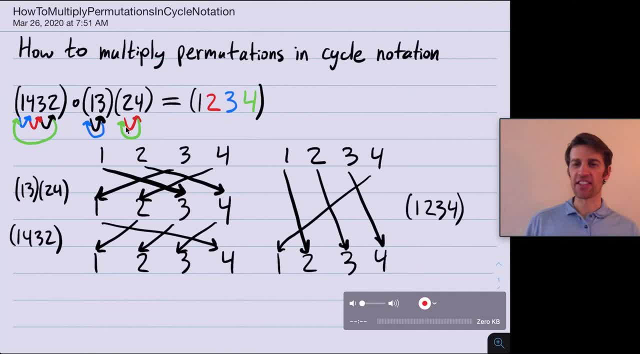 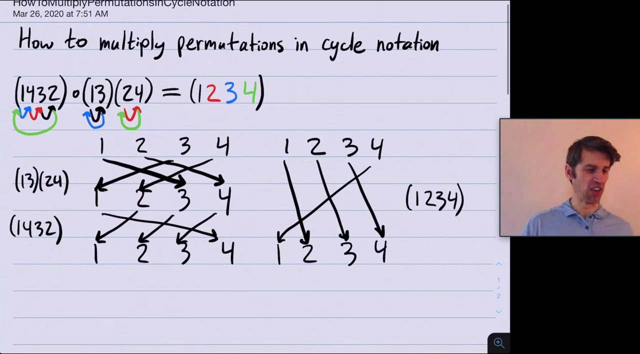 beginning, you'll see that each transition on the left hand side gets traversed exactly once. each each possible arrow on the left hand side appears exactly once, if you've multiplied this correctly. Okay, let me talk through a much harder and longer example. This is an 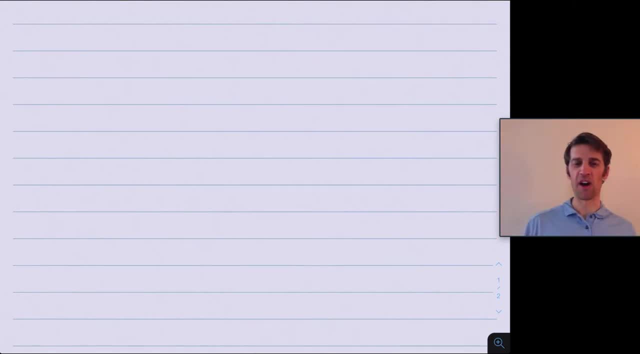 example, that is actually homework problem 1 on homework number 6 for my class Math 366, Introduction to Abstract Algebra at Colorado State University in 2020.. So the problem says the following: Write the permutation 1,, 2,, 4,, 3,, 8,, 9,, 2,, 3,, 6,. 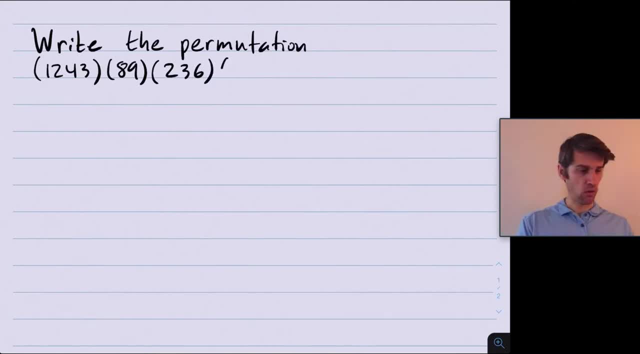 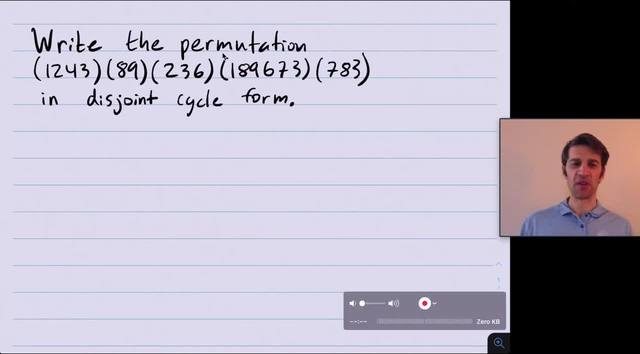 So disjoint cycle form means we don't want cycles that have elements in common right. This cycle has a 7, as does this one. We want to write this for the first time, So we're going to write this for the first time. 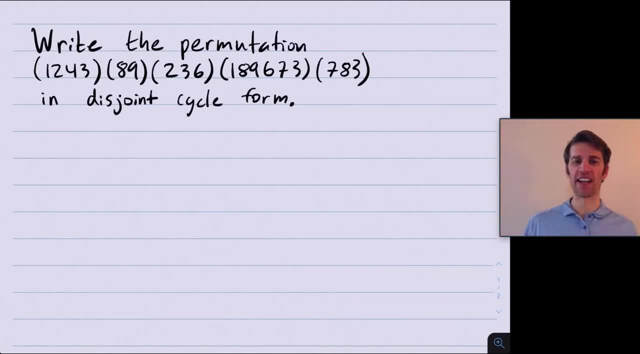 So we're going to write this for the first time. So we're going to write this for the first time As a product of cycles, where each cycle has distinct elements from any other cycle. The way to do this is just to multiply these permutations out and see what we get. 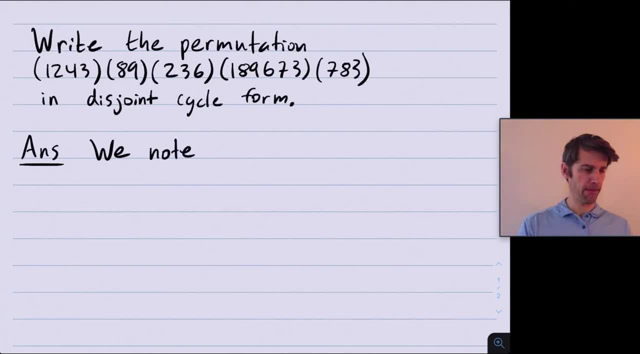 Okay, So I'm going to write down the problem again: 1, 2,, 4,, 3,, 8, 9,, 2,, 3, 6,, 1, 8,, 9,, 6,, 7,, 3,, 7,, 8,, 3.. 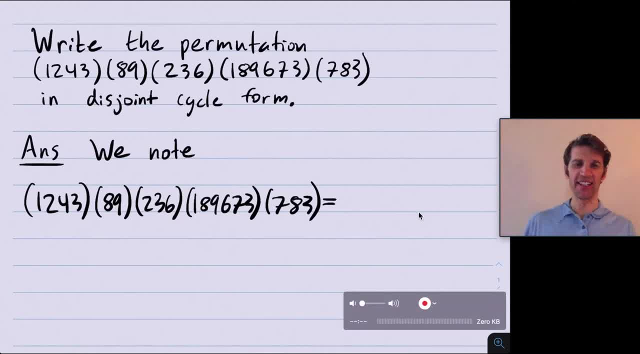 We'll be able to write out the answer right here. There's really not that much work to show. I'll try to draw some arrows as I narrate through this, But you don't need to draw those arrows. There's very little work to show as long as you understand the process. 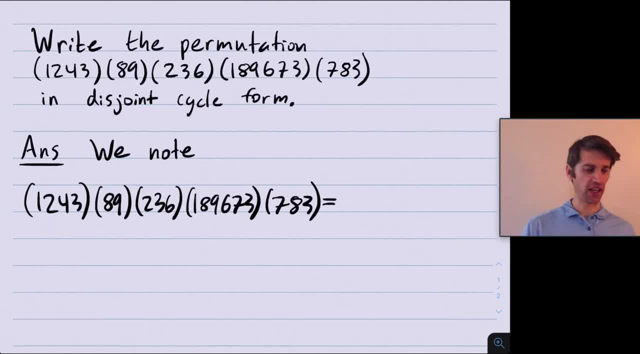 Okay, so to write a permutation in disjoint cycle form. first, you see where 1 goes. So 7,, 8, 3 doesn't move 1 at all. This next cycle, however, maps 1 to 8.. 2,, 3, 6 doesn't map 8 anywhere. 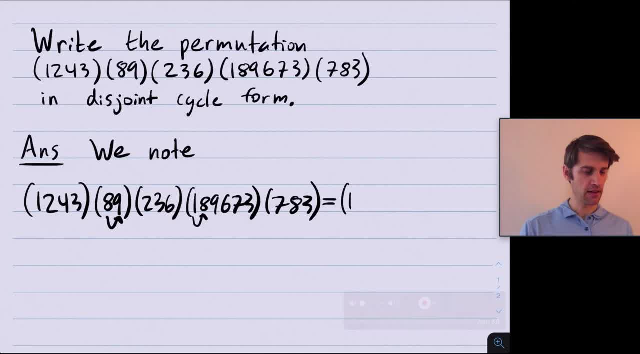 This next cycle maps 8 to 9. And then this doesn't map 9 anywhere. So in total, 1 is going to 8, and then to 9.. So 1 is going to 9. And that's why I put down a 9. next. 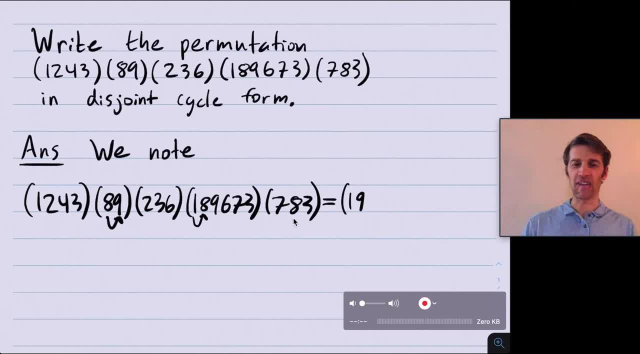 Now I want to see where 9 goes. So this cycle doesn't move 9 at all. This cycle moves 9 to 6.. This next cycle- 2,, 3,, 6, sends 6 back to 2.. 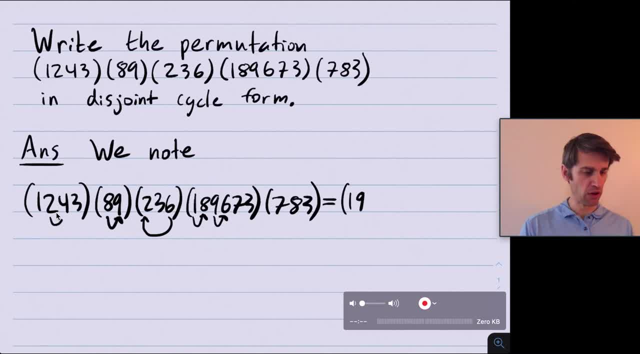 This cycle doesn't move 2, and this cycle moves 2 to 4.. So in total, 9 has been mapped to 6, and then to 2, and then to 4, so 9 is going to 4, and I write down 4 next. 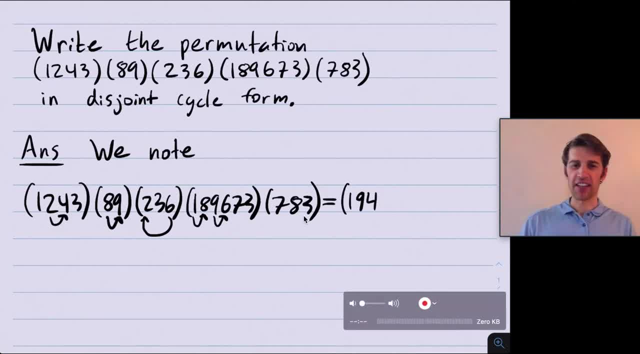 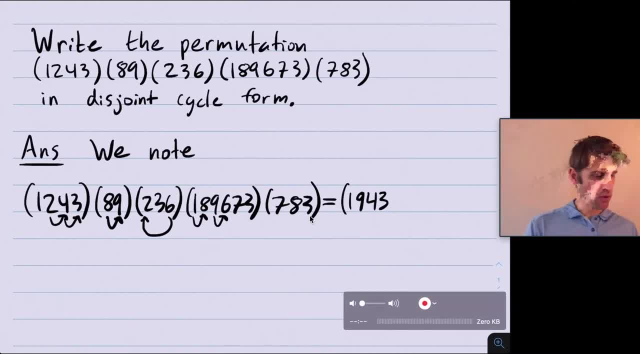 Where is 3 getting mapped? This cycle moves 3 to 7, and then this cycle moves 7 back to 3, and then this cycle moves 3 to 6,. the next cycle doesn't move 6,, nor does the last. 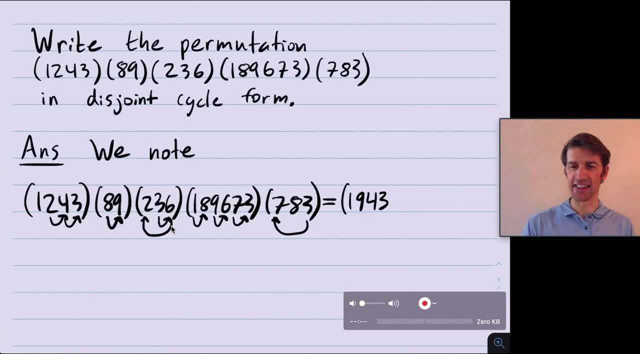 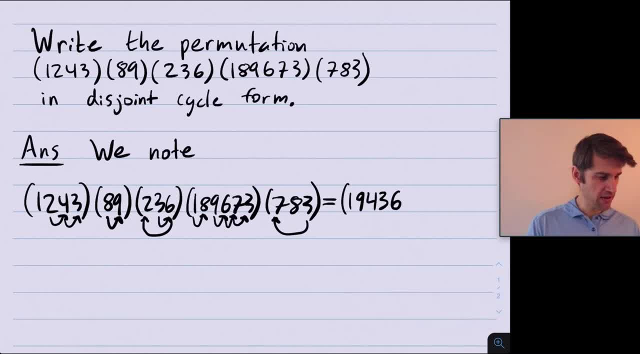 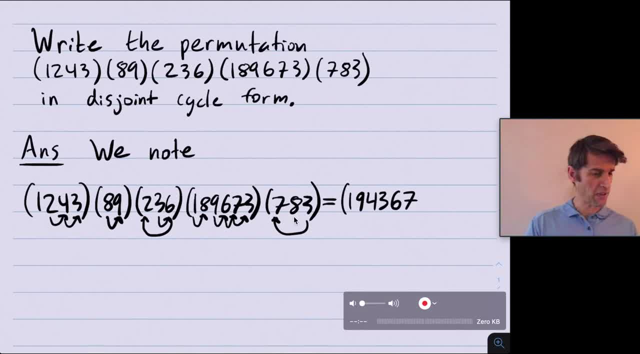 Where is 7 being mapped? 7 is being mapped to 8, which then 8 gets mapped to 9,, 9 gets mapped back to 8, and then this last cycle doesn't move. So 7 got moved to 8, because it went to 8, and then to 9, and then back to 8.. 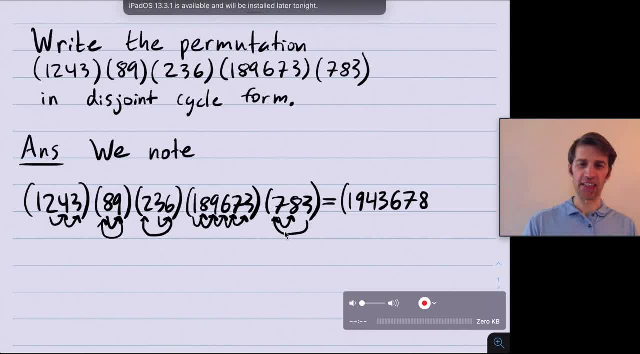 Alright, let's see where 8 gets mapped. So this cycle moves 8 to 3, and then this cycle moves 3 to 1, and then 1 doesn't get moved by either of these two cycles, but here 1 gets mapped to 2.. 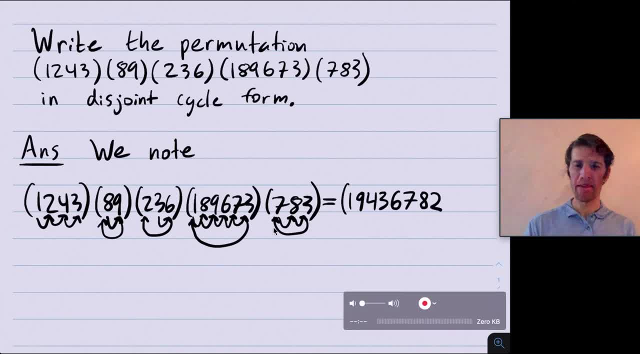 So 8 is being mapped to 2,, because it went to 3, and then to 1, and then back to 2.. And now let's see where 2 goes. This cycle doesn't move 2,, nor does this one. 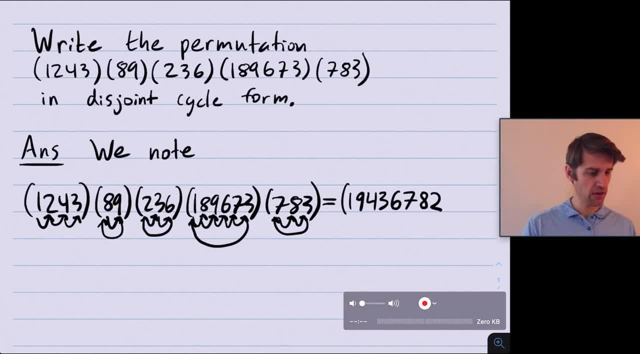 This cycle moves 2 to 3, and then 3 gets moved back to 1.. So 2 is going to 1.. I noticed that 1 was the start of this cycle, So I denote that by closing this parenthesis. Okay, so I've told you where 1,, 2,, 3, and 4 go. 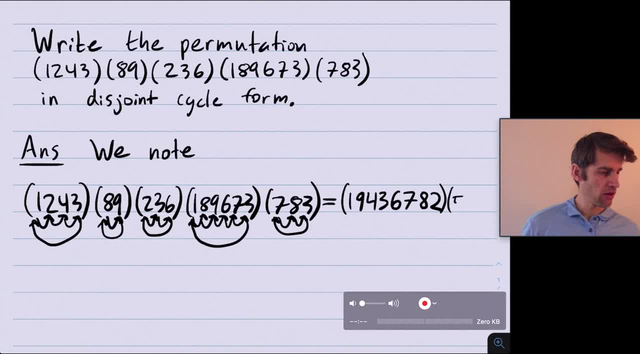 I haven't told you where 5 goes. Where does 5 go? Well, this cycle doesn't move 5, nor does this one, nor this one, nor any of the cycles. So 5 just gets mapped to itself. I've told you where 6 goes, where 7 goes, where 8 goes and where 9 goes.